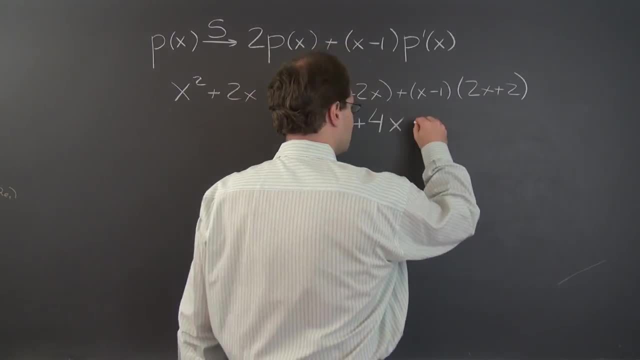 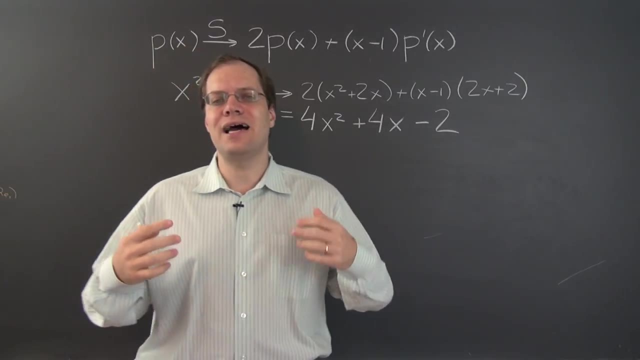 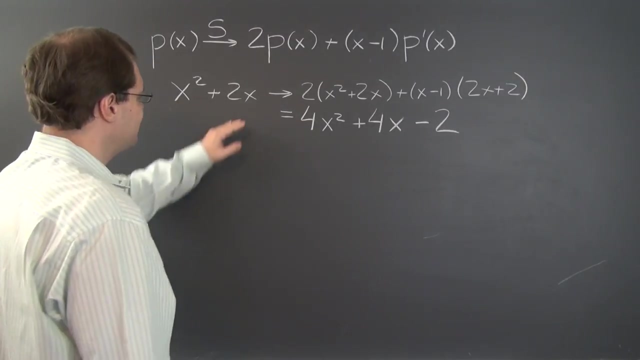 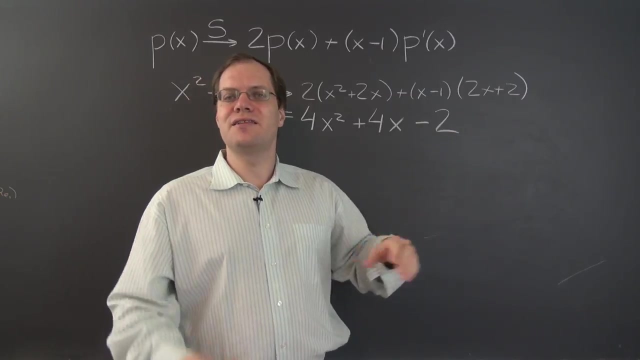 And the only term that's remaining is the constant term, which is minus 2.. So that's what this silly linear transformation does. Now let's analyze it in component space, which is of course done by choosing a basis, decomposing this vector with respect to that basis and multiplying it by the matrix, its components, by the matrix that represents this linear transformation. 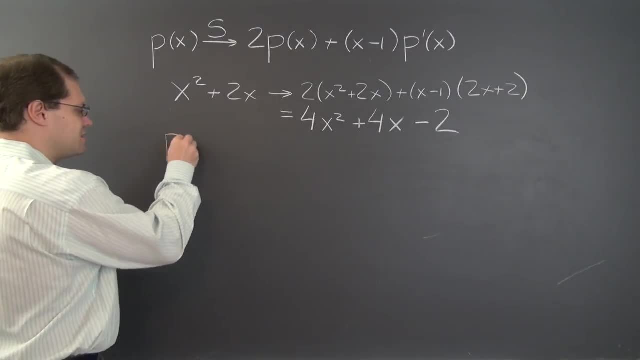 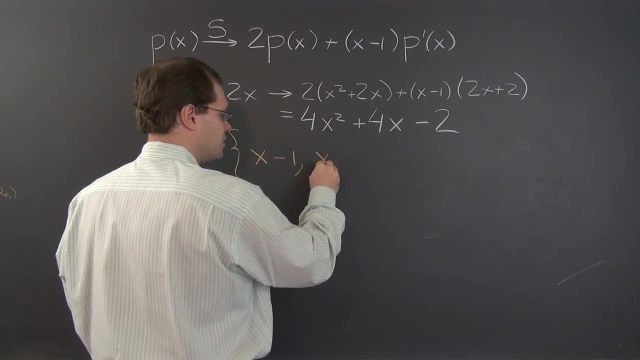 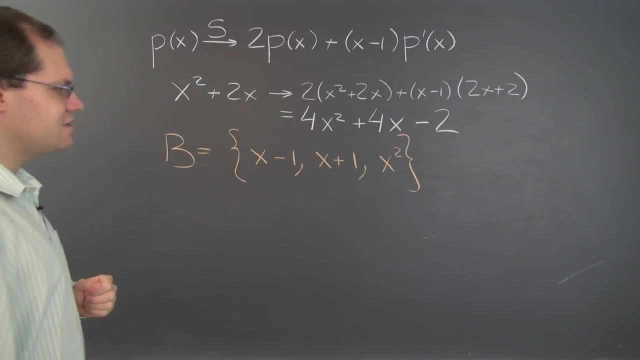 So quite a bit of work ahead of us. Let's start by picking a basis. How about x minus 1,, x plus 1, and x squared Alright, And we'll construct the matrix s squared Alright S, sub b right here. 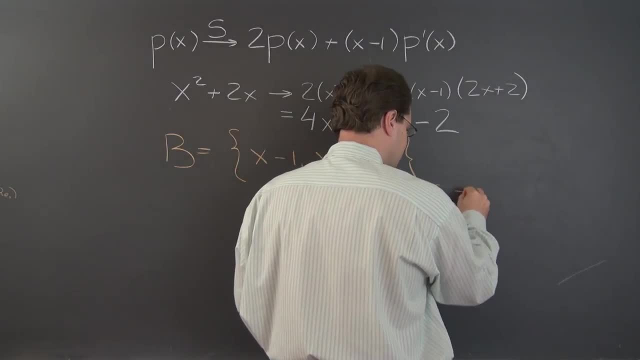 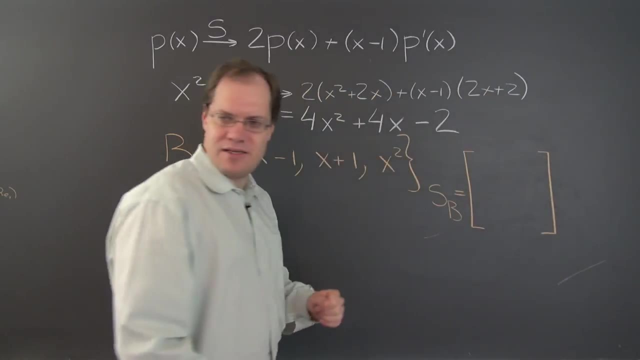 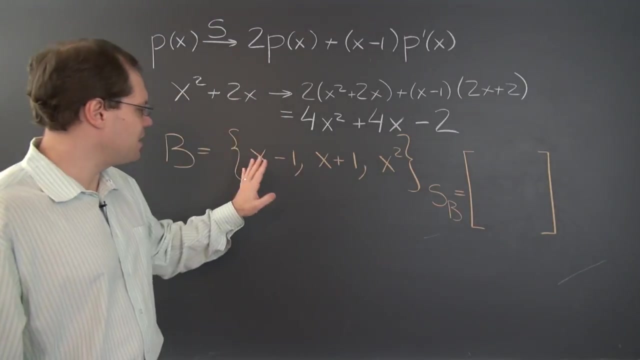 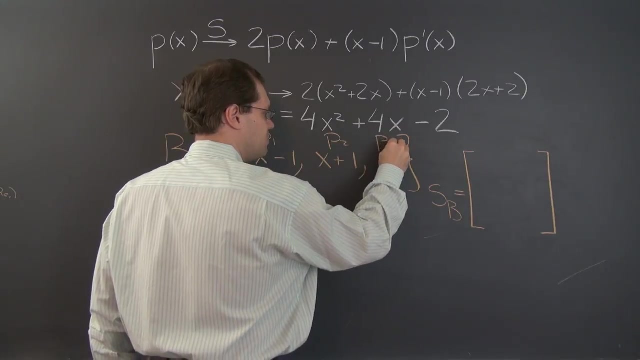 Let's make sure that it will fit. S sub b equals it's 3 by 3, because we're dealing with a three-dimensional space here. Okay, And here we go. The first column will correspond to the first element, So let's call this p1,, p2, and this will be p3.. 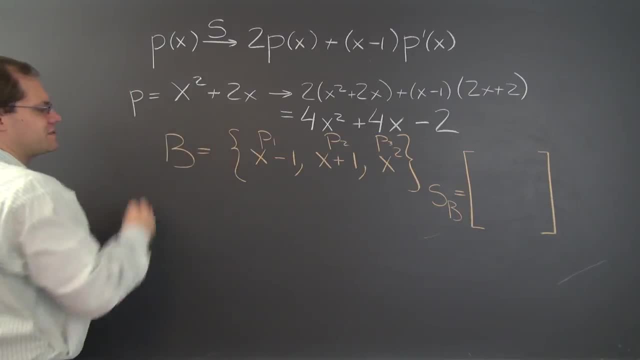 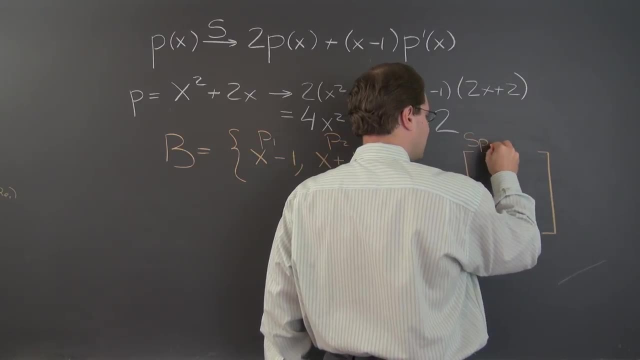 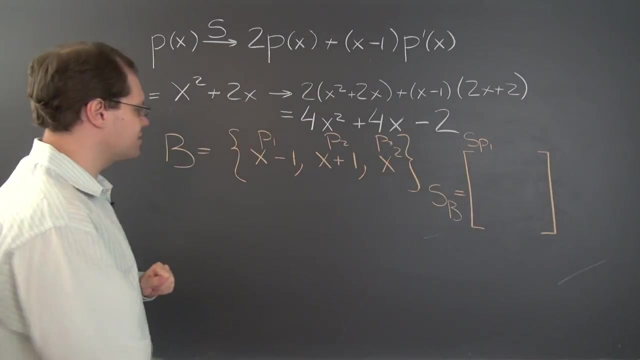 And this polynomial we'll call p, p of x, p. So the first column will have s of p1 in it, More specifically the coefficients of s of p1 with respect to the same basis. So we have to compute this transformation applied to this vector. 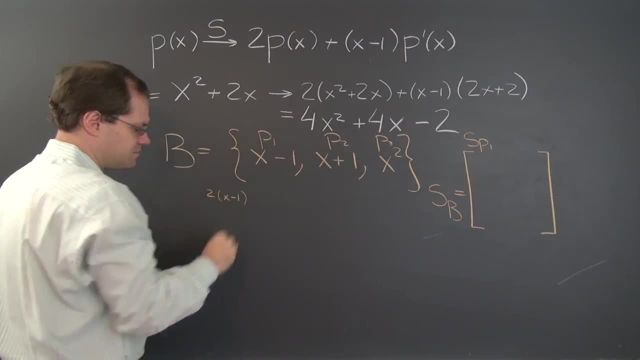 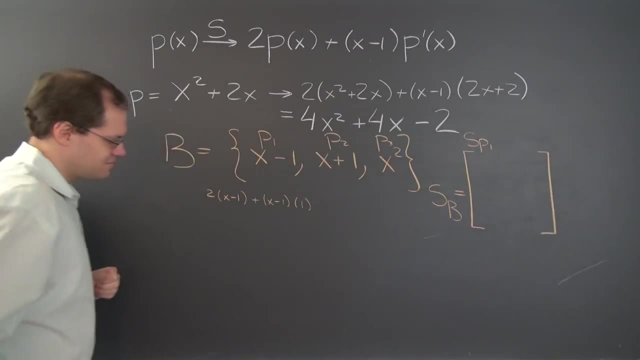 So it'll be. I don't want to waste too much space on it. twice itself, Twice itself Plus x minus 1 times its derivative. There you go, And the answer is 3 times x minus 1.. Look at that. 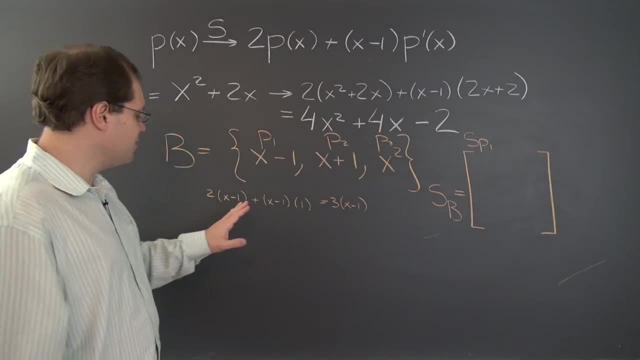 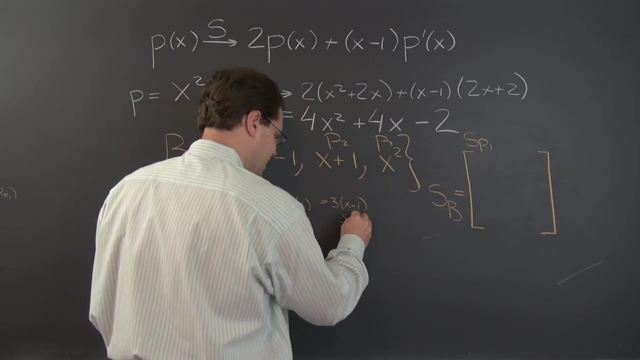 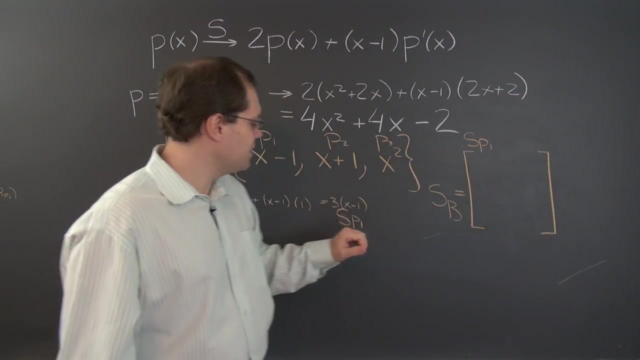 We found an eigenfunction of this transformation 3 times the original function, And now we have to decompose the result. This right here is s of p1. Capital S of p1. And now capital S of p1 needs to be decomposed. 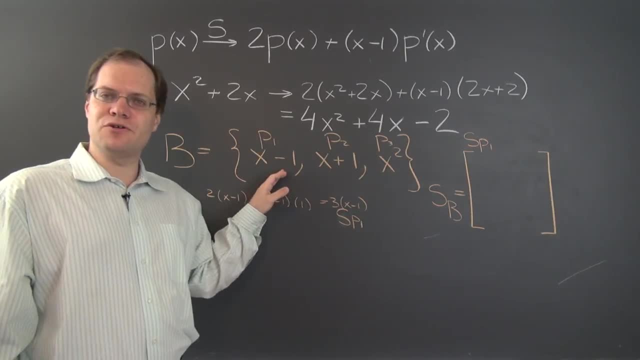 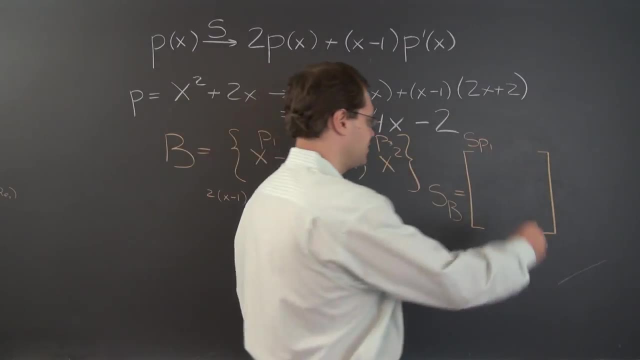 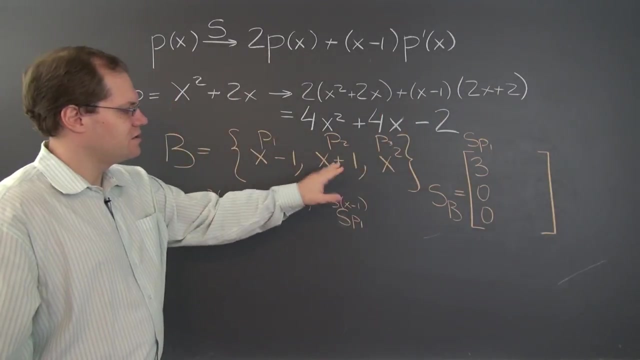 with respect to the same basis And, of course, the coefficients are 3, 0, 0.. And that's the first column of this matrix: 3, 0, 0.. Great, Now let's move on to the second one, which is rather easy. 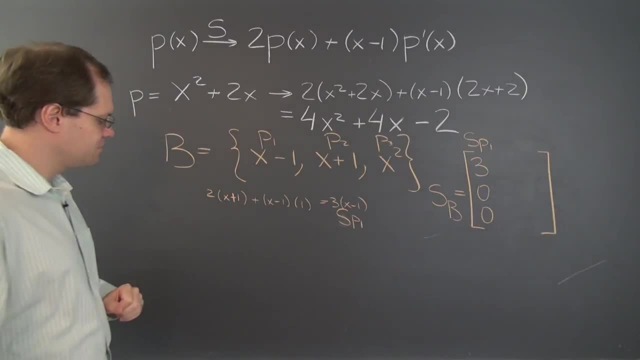 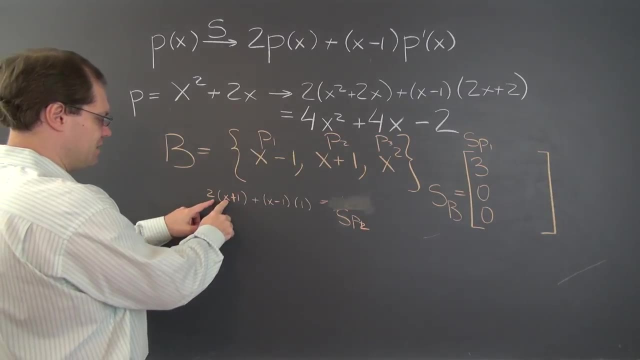 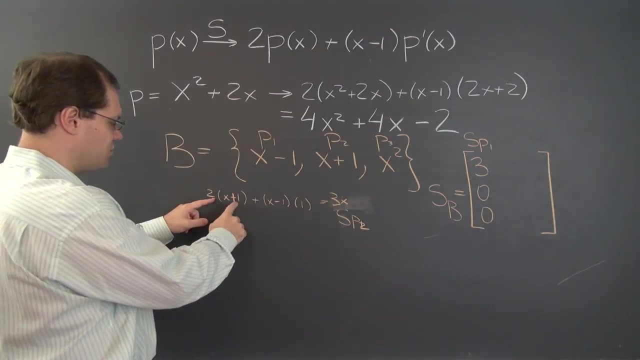 This becomes x plus 1.. So now we have to be a little bit careful. This will be in a moment s of p2. And it'll be 2x plus x, 3x And then 3x plus 1.. 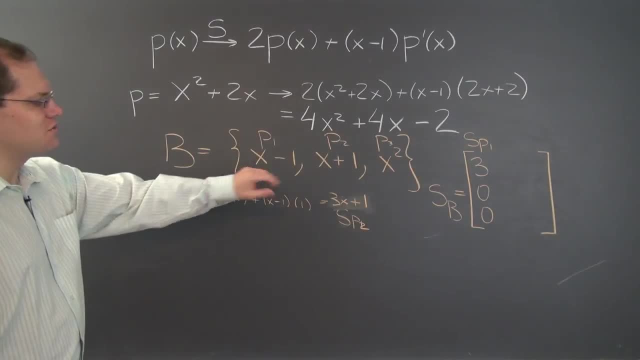 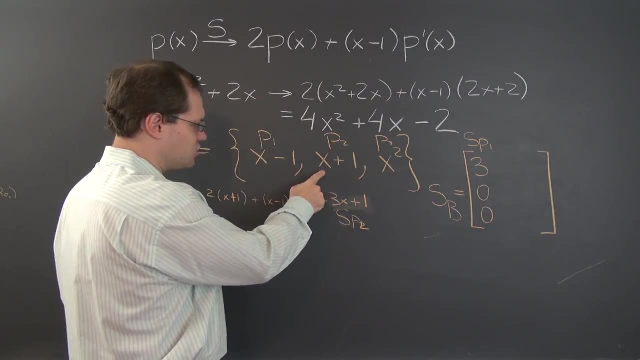 I was already beginning to decompose it in my mind with respect to this basis. All right, So not so easy, but hopefully not so difficult. So I'm thinking we'll take 2 of this one and subtract: Nope, Not so easy. 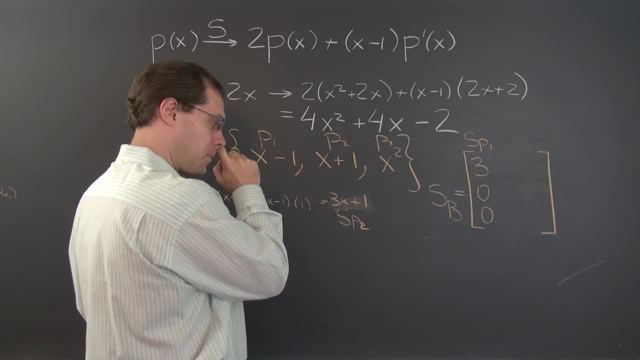 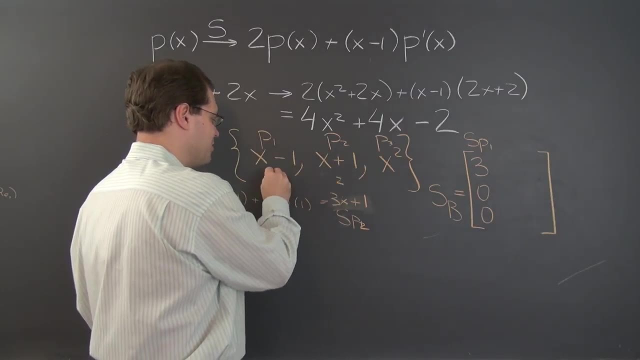 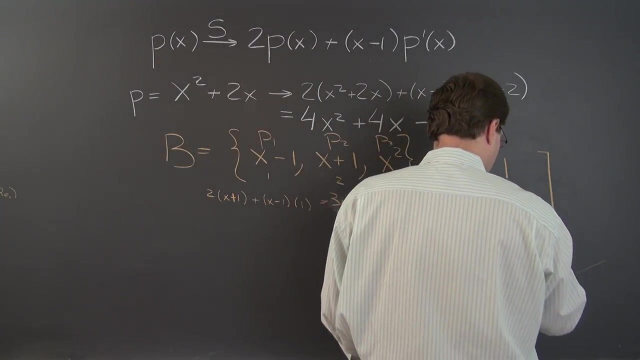 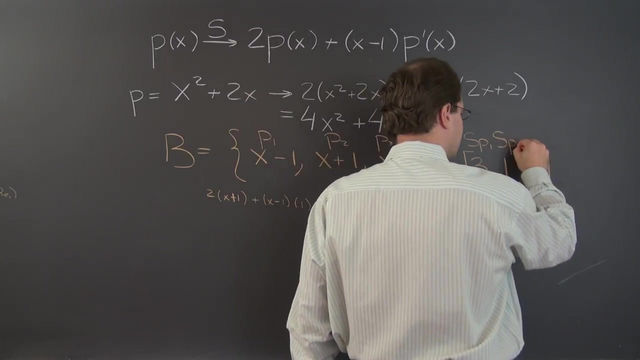 That was right. 2 of this polynomial and 1 of this polynomial does the trick. So 1, 2, 0.. 1, 2, 0.. Great, Finally, the same, the exact same thing. This is s of p2.. 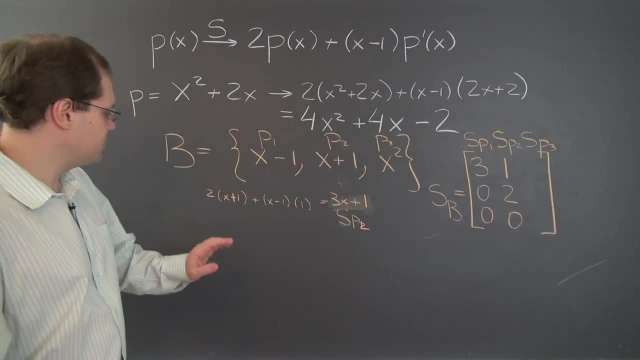 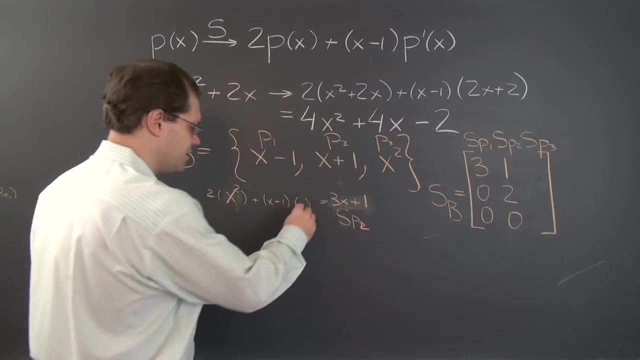 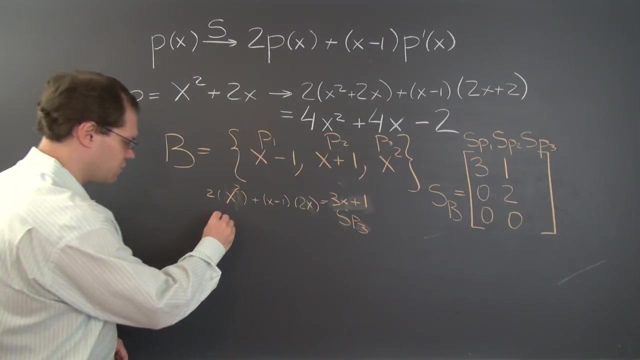 The exact same thing for s of p3. So p3 equals x squared, So it's 2 times x squared times x, minus 1 times its derivative, And that, in a moment, will be s of p3. So we have 2x squared. 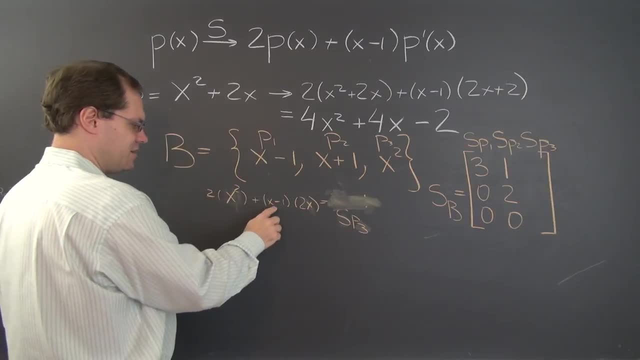 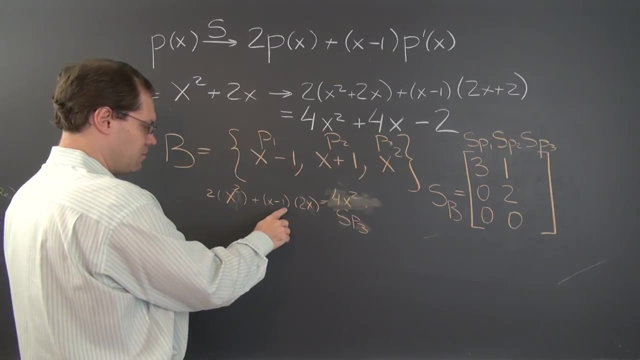 Nope, not 2x squared. So 2x squared from here and 2x squared from here. So 4x squared: No x here, Minus 2x, 2x squared. 2x squared, So 4x squared. 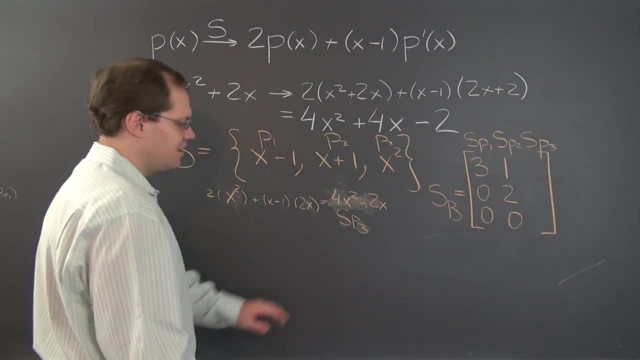 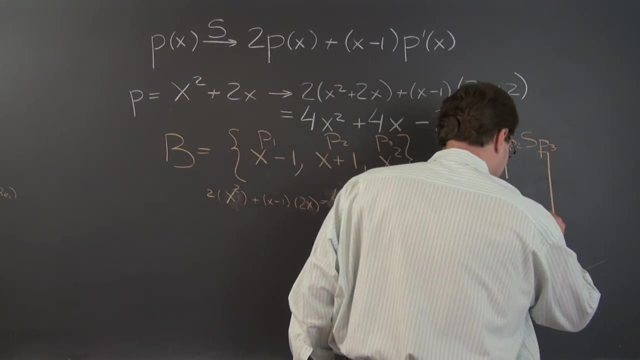 And then minus 2x, Minus 2x, And we now have to decompose this polynomial with respect to the same basis. So the one part that's obvious is that this gets a 4. And what's left is having to do minus 2x. 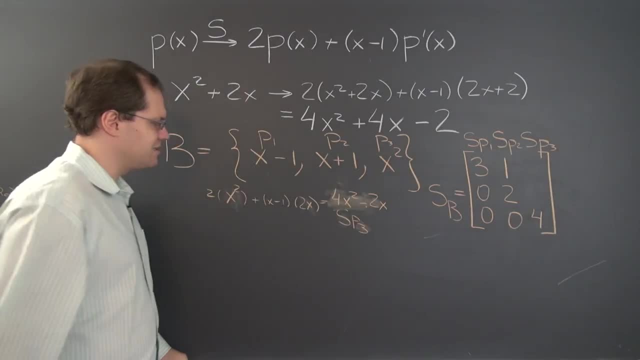 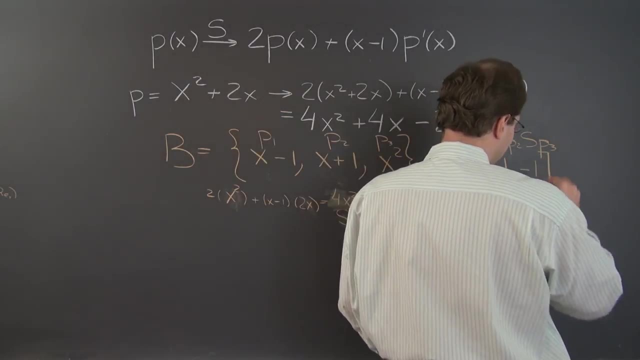 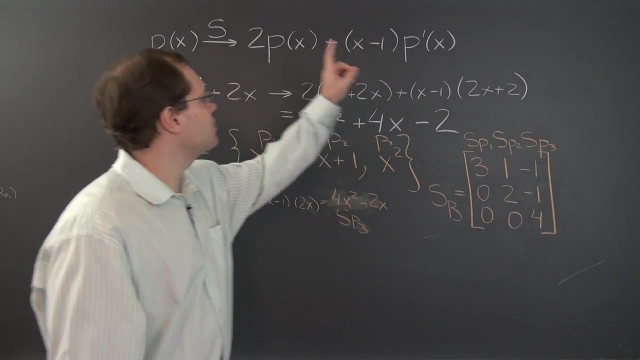 Which, of course, is minus this, minus this. So minus 1.. Minus 1.. Minus 1. 4.. Minus 1. Minus 1. 4.. And we have accomplished the task of calculating the matrix that represents this silly linear transformation with respect to this basis. 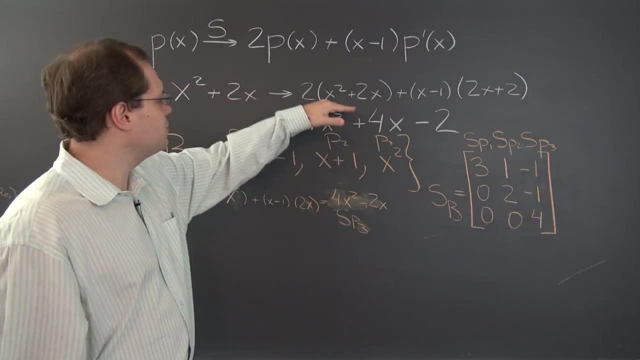 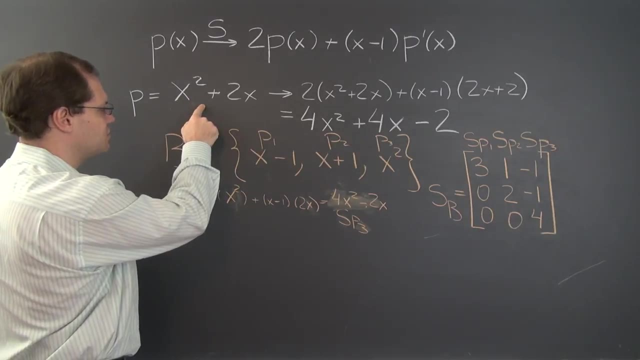 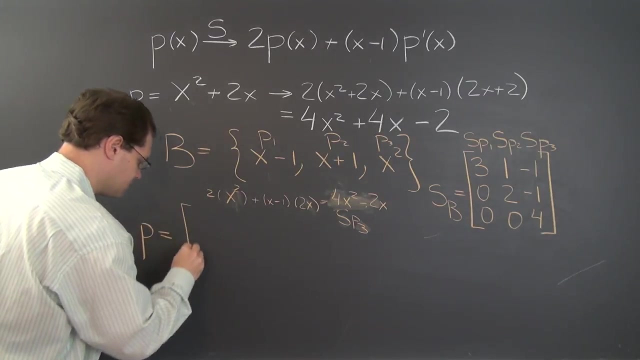 Now let's just make sure once that it works by using this polynomial, for which we know the answer, And our first task that we need to accomplish is to decompose this polynomial with respect to the same basis. So we have P equals, So of course, it's 1 of the last one. 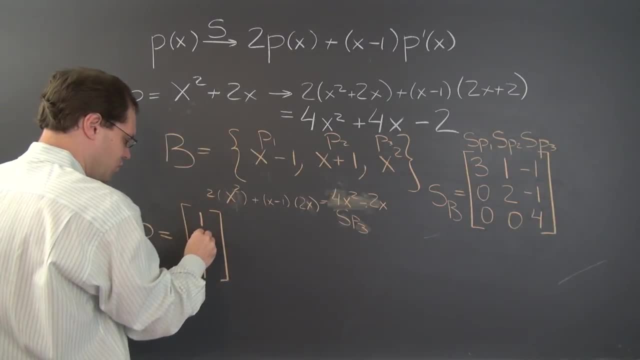 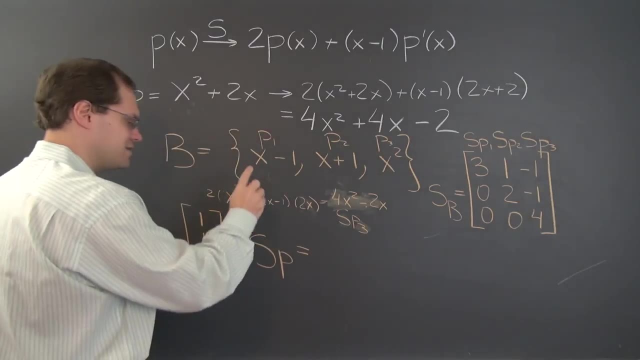 And the sum of these two, So 1, 1, 1.. 1, 1, 1.. Very nice, And so, in order to evaluate S of P, we need to multiply this matrix by 1, 1, 1.. 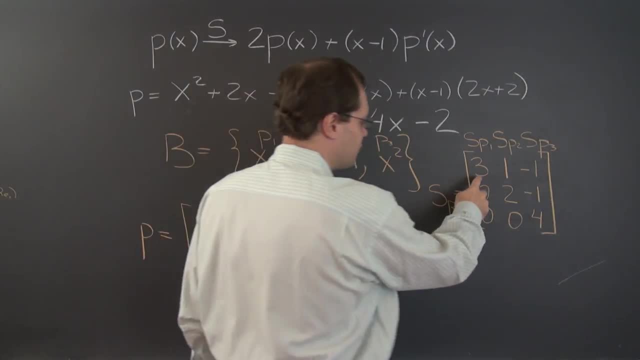 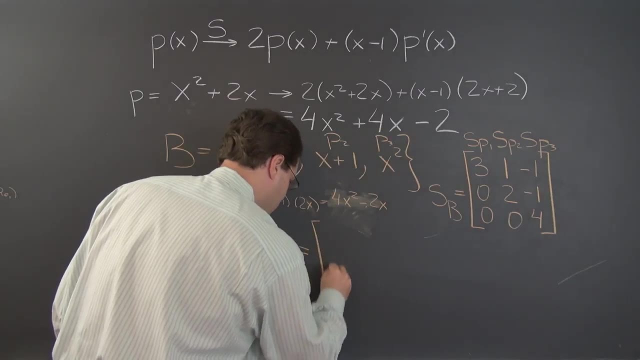 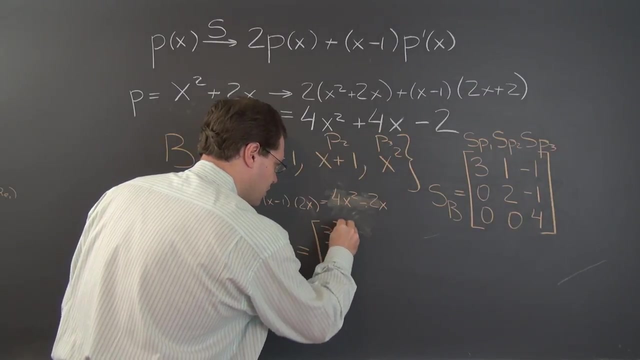 And of course, this will sum up each of the rows, So we'll have 3, 1, 4.. 3, 1, 4. 3.. So this is with respect to the basis B: 3, 1, 4.. 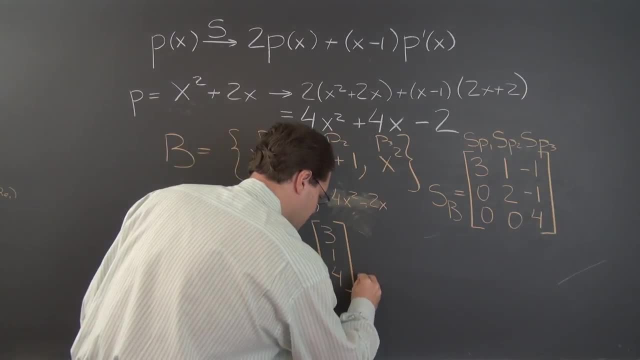 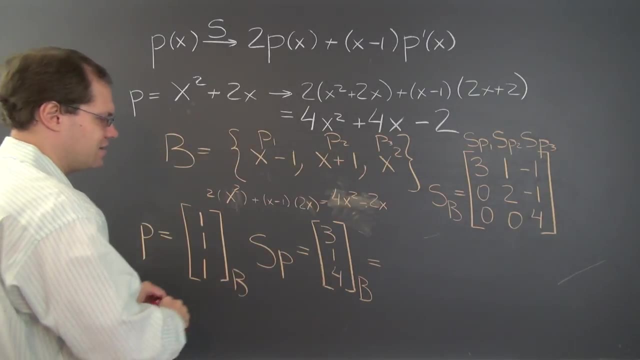 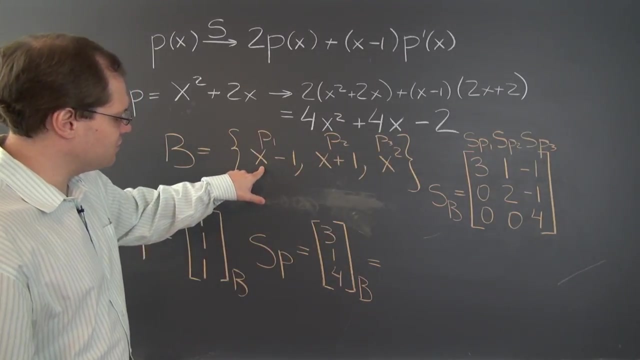 3, 1, 4.. Also, with respect to the basis B, And let's see what this combination represents, And I'll erase this line because it was just workspace, All right. So what we need to do is add 3 of this plus 1 of this, plus 4 of this. 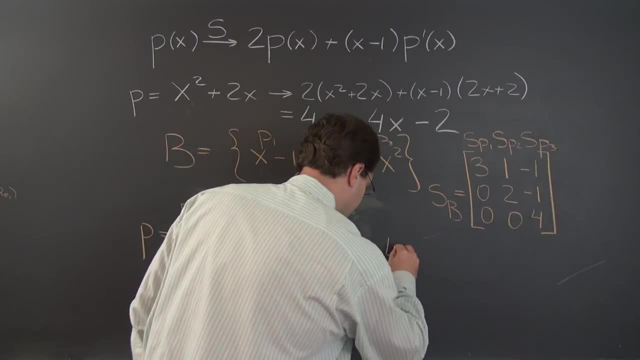 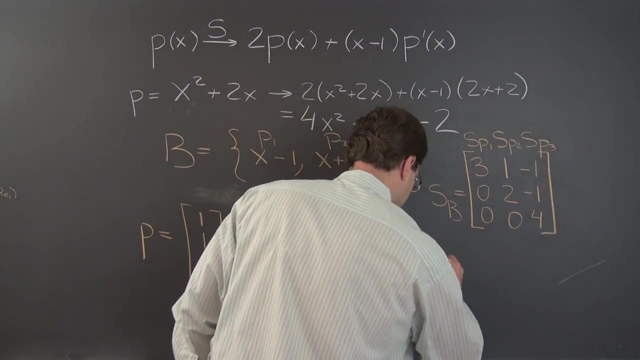 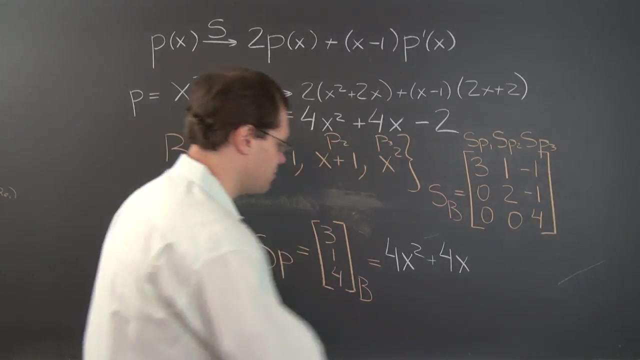 So we'll have 4x squared, 4x squared plus 4x, And then this will give us minus 3 and this will give us plus 1. So minus 2.. So 4x squared plus 4x. 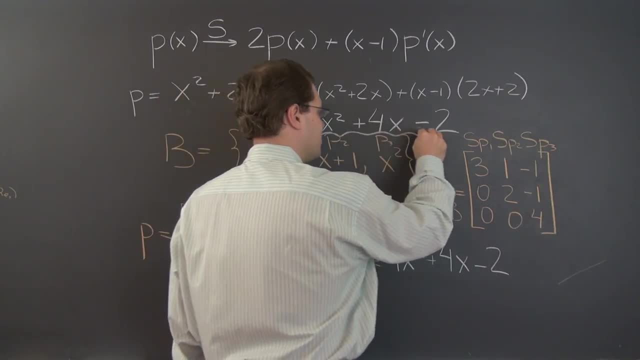 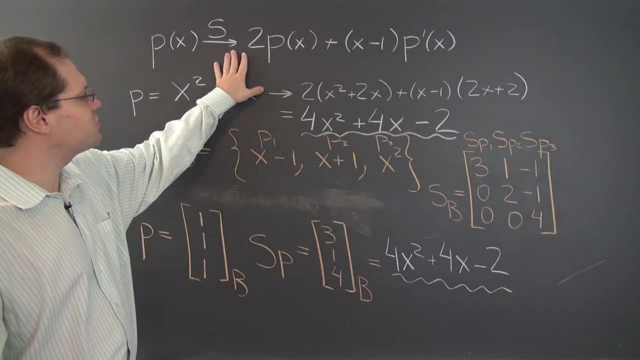 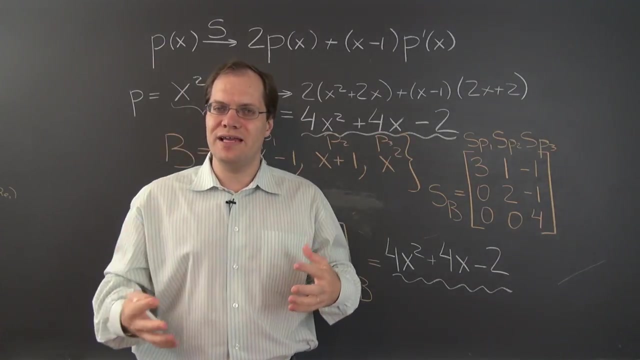 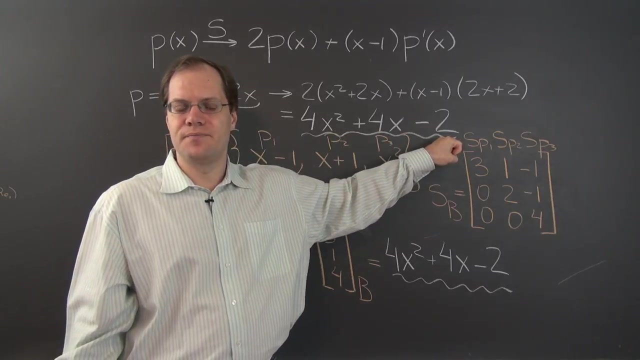 Minus 2.. The exact same polynomial as before. So just to review, what we started out doing is evaluating this transformation applied to this polynomial right here And when. we did it without the use of any basis or any component spaces. we evaluated it directly and got this answer. 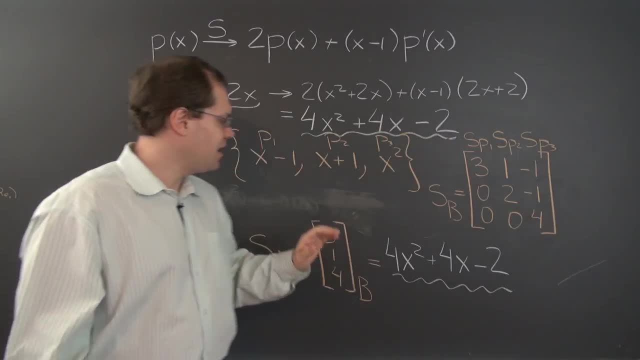 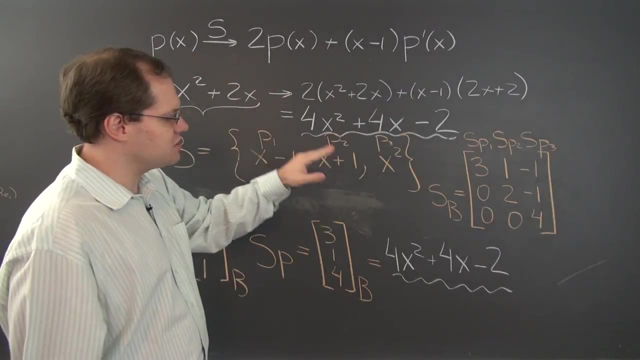 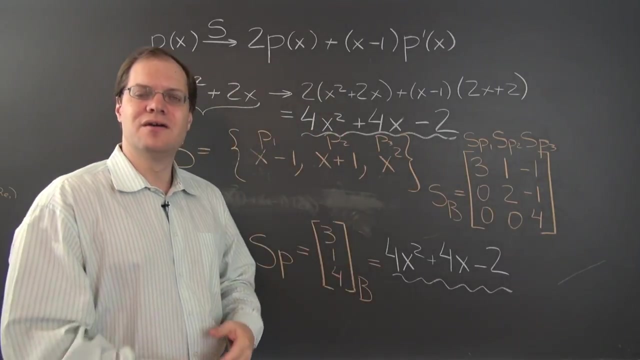 Then we made a foray into the component space. After that, we chose a basis, Constructed the matrix that represents this linear transformation. with respect to this basis, Which is done a column at a time, We still haven't fully justified why it works.